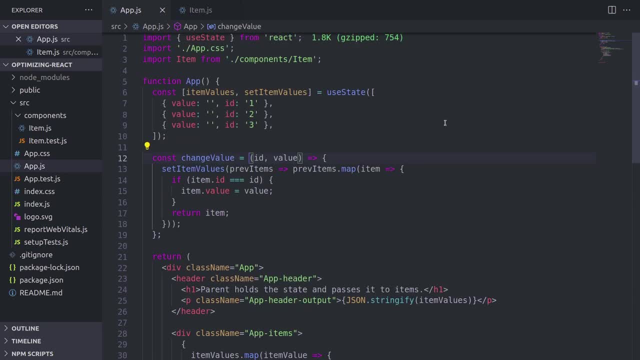 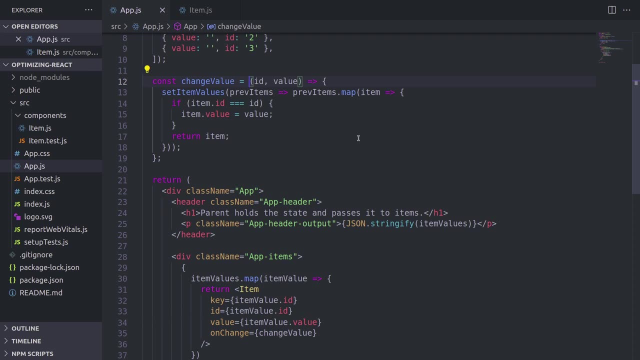 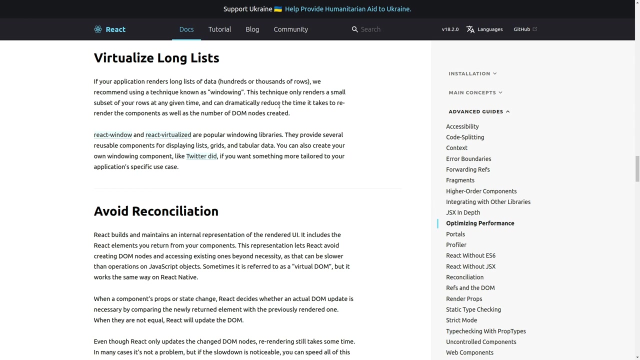 All right guys, before we dive deep into code and start optimizing our app, I would actually suggest going to React documentation to see what they actually recommend us when it comes to optimizations. So in the docs, under advanced guides, we have this section called optimizing performance and there 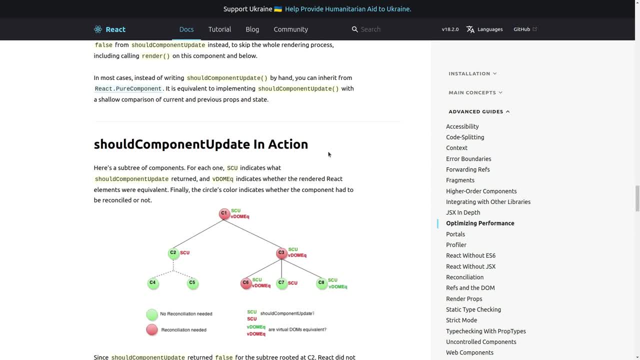 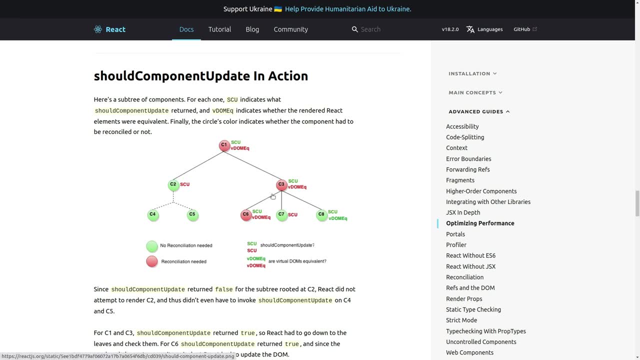 they give different techniques on what to pay attention to when it comes to optimizations, and they also give you a lot of information about how to optimize your app. So let's get started, And this section is what we're going to be focusing on. How does React re-render its children and how 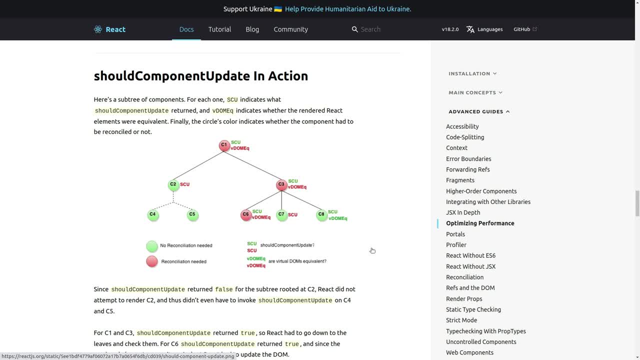 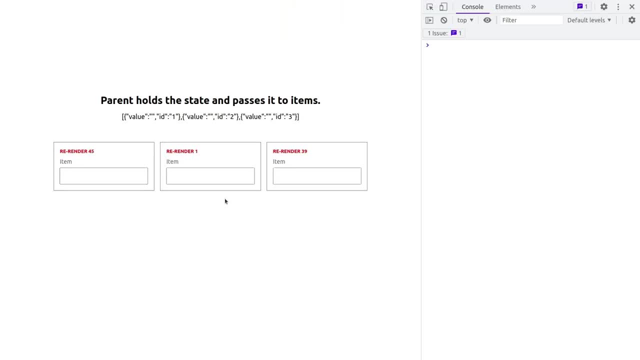 does it decide to do so. I would actually suggest going through this content to be familiar with it. Now, going back to our example app, I gotta say that it's unfortunately not performant. We have this state in the parent and we're rendering three children boxes with input fields As soon as I 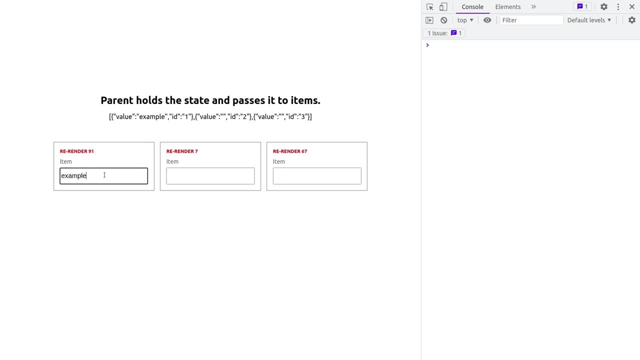 start typing something, it's going to propagate back to the parent and update the state. But look at these re-render numbers. These are simply random numbers that I put there, but as soon as I start typing in one of the boxes, all three start changing. It means they're being re-rendered. 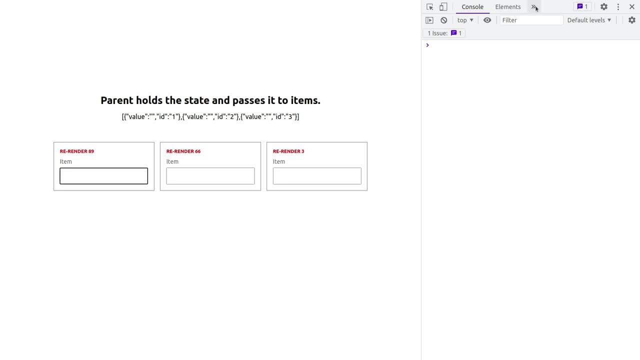 To kind of prove that we need to have React DevTools installed. and I have it and I'm going to go to the profiler. In the profiler settings I'm going to turn on this checkbox called highlight updates when components render. And now it's going to give us a. 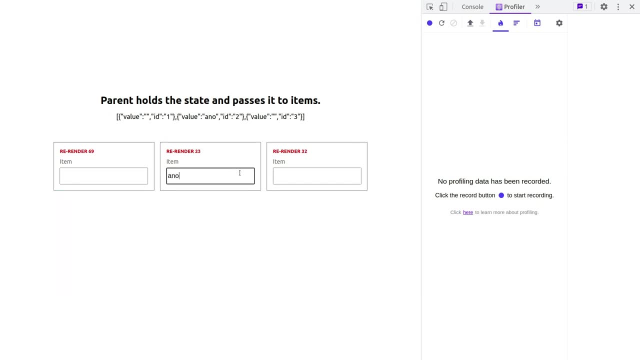 really nice representation. So I start typing something. As you can see, all three boxes have highlighting. It means the components is literally being re-rendered every time I type a letter, So obviously that's not good. Why should other components get re-rendered when I'm typing? 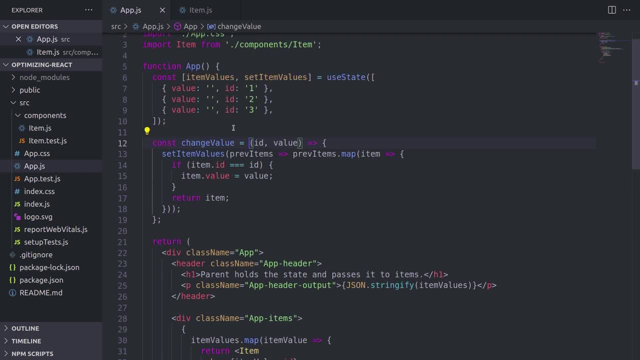 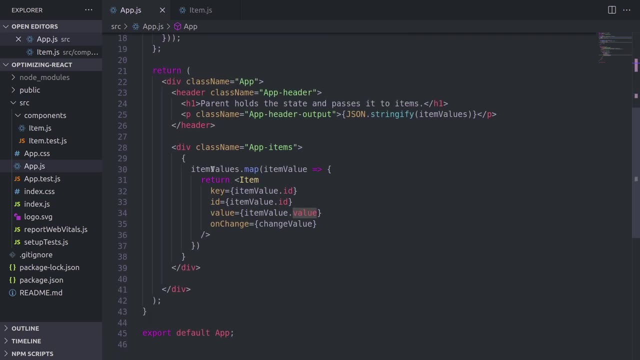 only in one of them. Let's go to the code. In the code, our parent component is called app and it holds the state for three items that are being looped through. The loop is here And we are creating an item component and passing different props to it, such as key ID value. 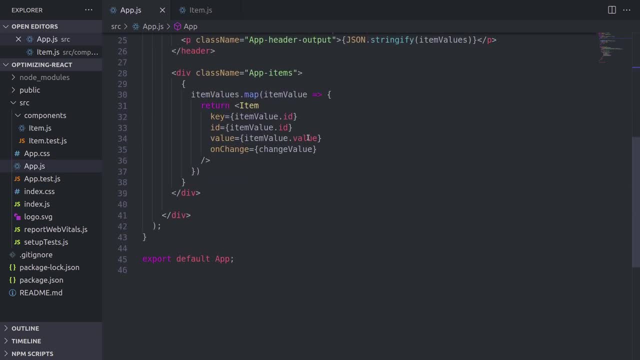 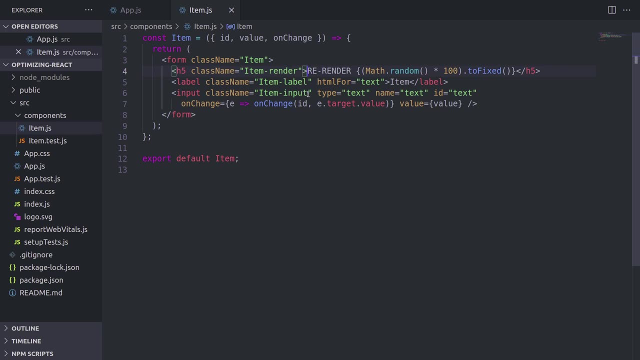 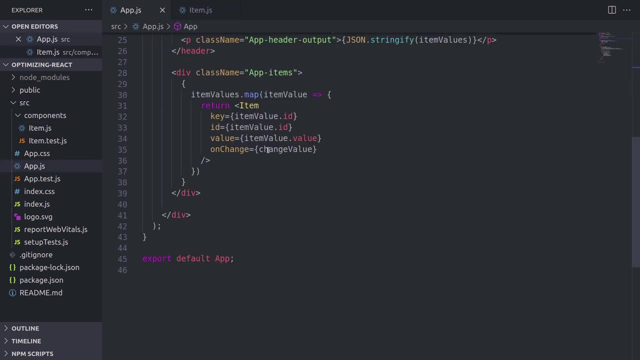 So ID is here and we're also passing value And we're also passing a handler function as a prop In the itemjs, which is basically the child. we have this re-render that I told you about, But we also have this on change function, which is going back to the parent, and we then fire change. 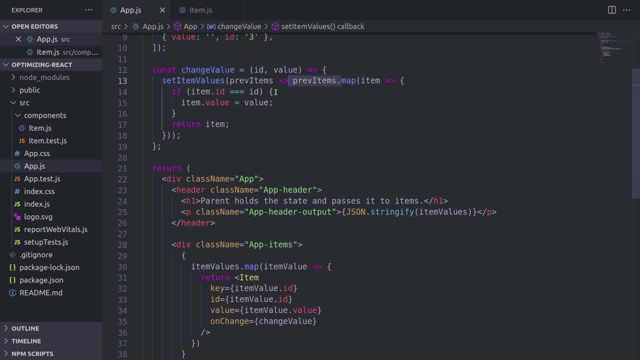 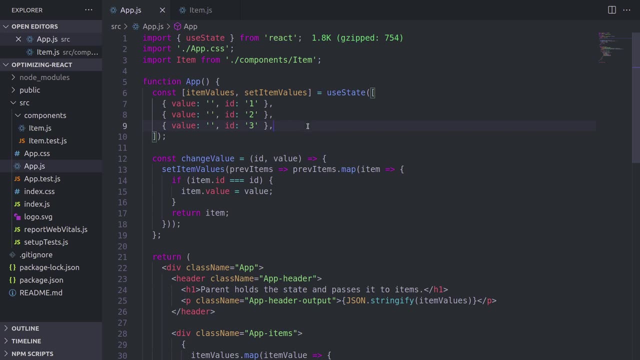 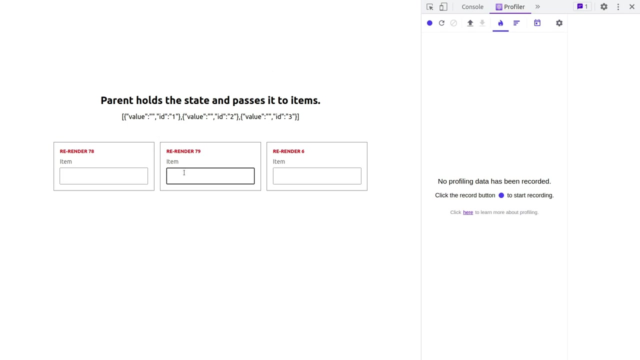 function, which is basically updates the states with this set item values. So there we map, We look for the exact the same ID that triggered the input change and we're updating its value. Pretty simple so far, right. So let's take a closer look at what's happening here. So I'm gonna start changing the 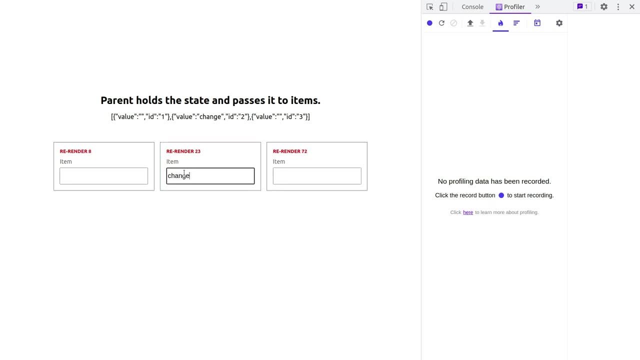 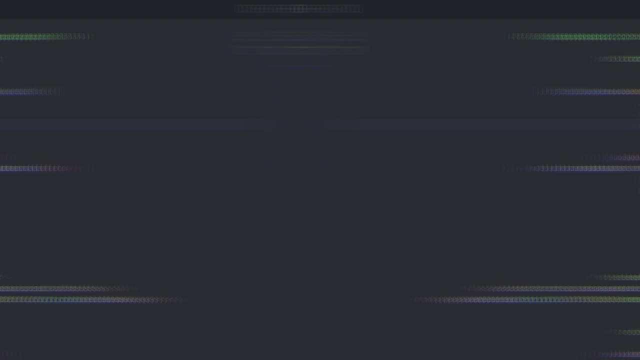 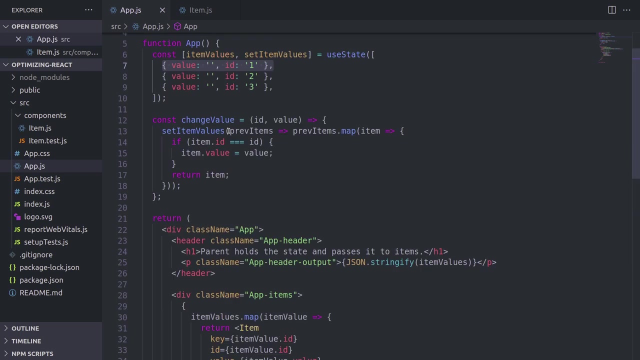 value in the middle box. So, as you can see, the state also changed, but apparently it triggers re-rendering in two adjacent boxes. Why? Why is one of the objects is changing and we are re-rendering all three objects, meaning all three items here? Well, one of the most common misconceptions about React is that it's 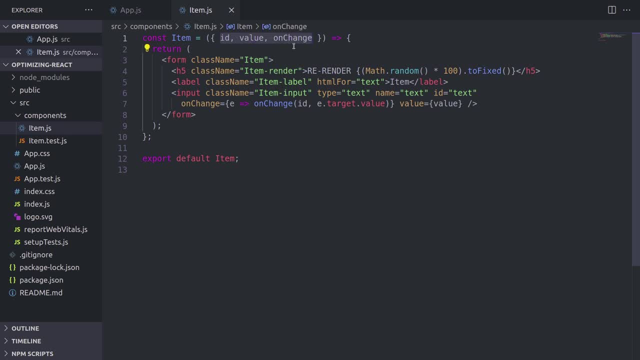 not going to re-render children unless these three props have not been changed. In fact, that's not true. As long as the parent gets re-rendered, it re-renders all of its children recursively. So that's what's causing our performance issue. To alleviate that, we can. 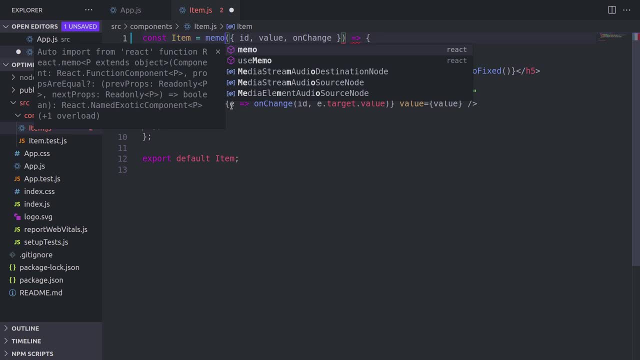 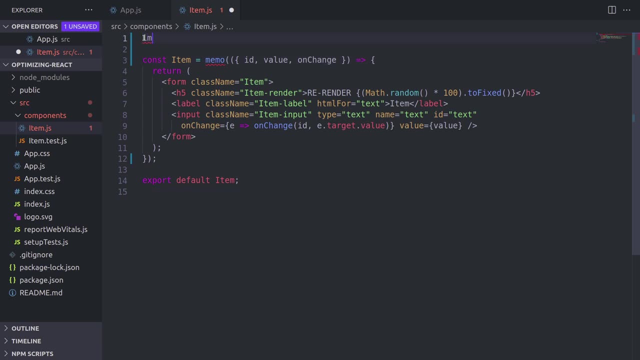 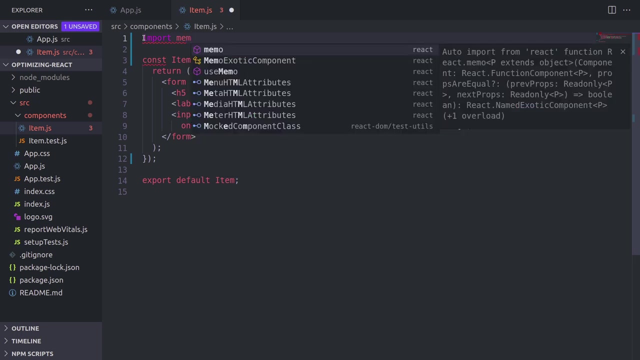 use this memo function. So we simply wrap our component in memo. Memo function simply memoizes this component. Memoizing means that it's going to remember what the previous prop was and if it didn't change then it's not gonna re-render our itemjs. 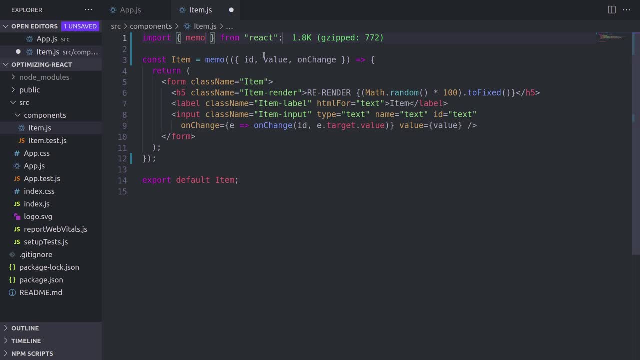 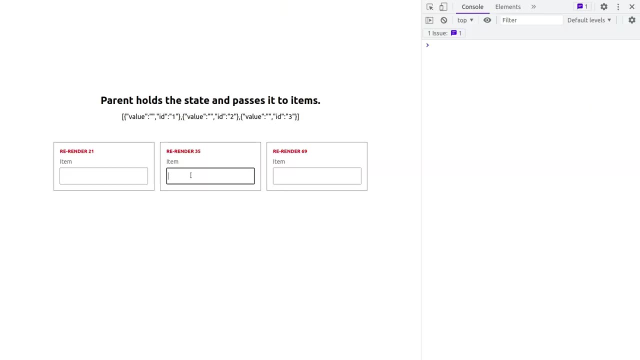 and we imported it very simply and I think that should fix the problem. Let's go back to the app Refresh and start typing again and hope that it works Well. I start typing example, but you see that the components are still getting re-rendered. 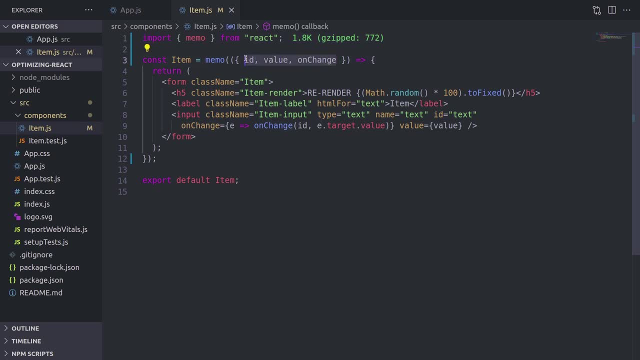 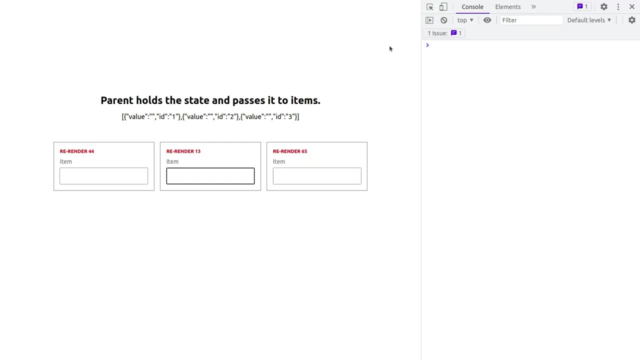 Hmm, something's wrong here. I wonder why. So it means one of these props still changed. So the parent still changed one of these props, but why It should have been memoized. Well, let's dig deeper. Let's go to the profiler again. 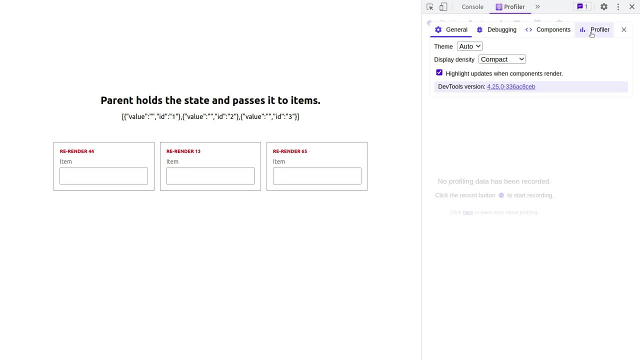 and now turn on this thing: under profiler- and it's called record- why each component re-rendered while profiling very self-explanatory. Let's start recording And as we record, I'm gonna change the value in this middle box. So I am editing and let's stop the recording. 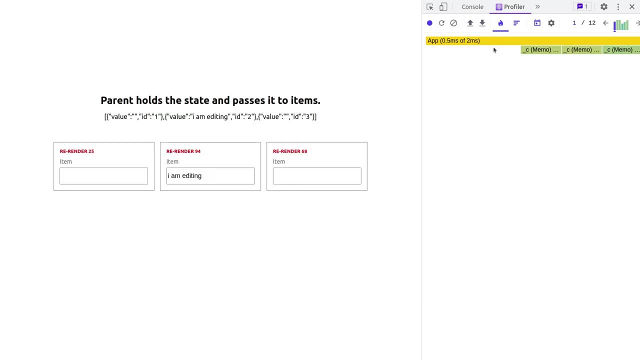 and see what we have. So we have these three boxes that have been changed. So let's start from the middle box. Why did this re-render? So props changed value. Obviously I changed the value. All right makes sense. And on change, let's look at the first box. 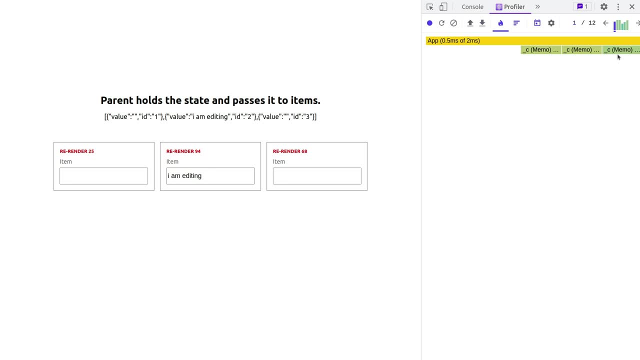 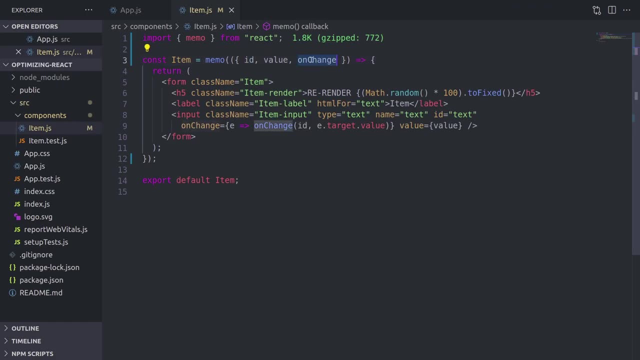 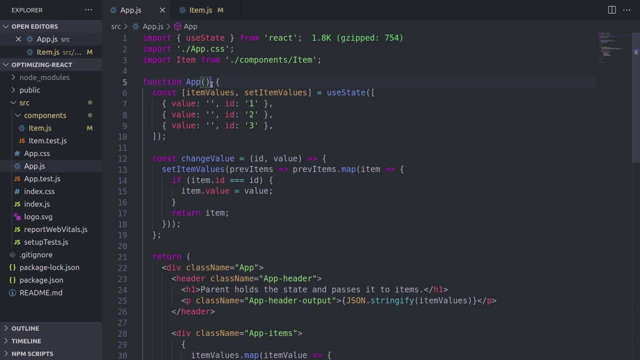 Props changed on change. That doesn't look right, And the same here. So, going back to the code, it seems like this: on change: prop got updated, Although these two guys are fine. So let me explain why. When the state in the parent gets updated, React recreates the whole component. 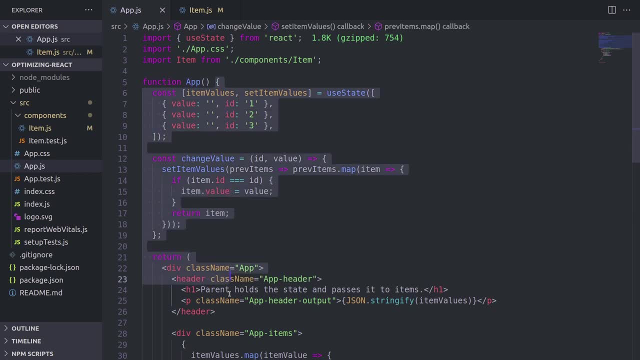 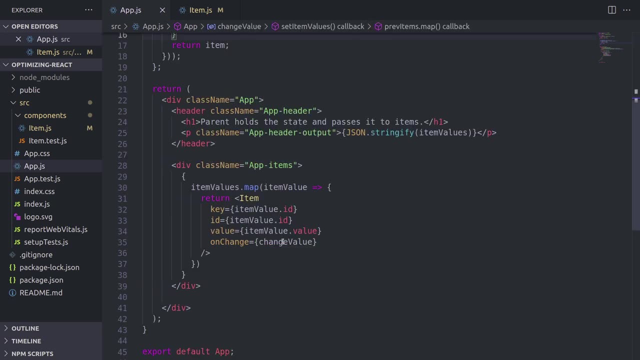 Basically it re-renders it and whenever it gets re-rendered this changed value function gets re-created. So imagine it's recreated. How does the child know that this is the same function that was passed before the re-rendering? 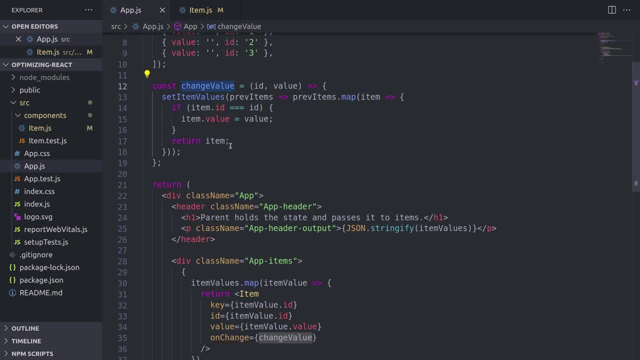 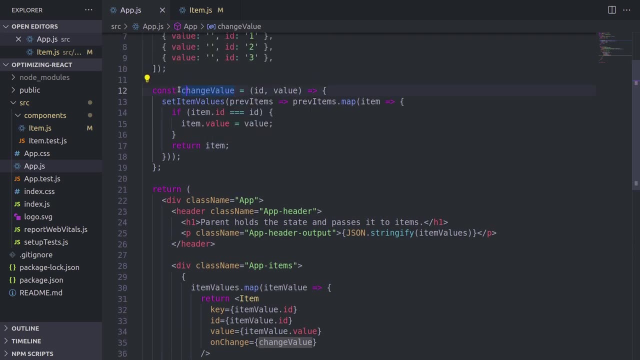 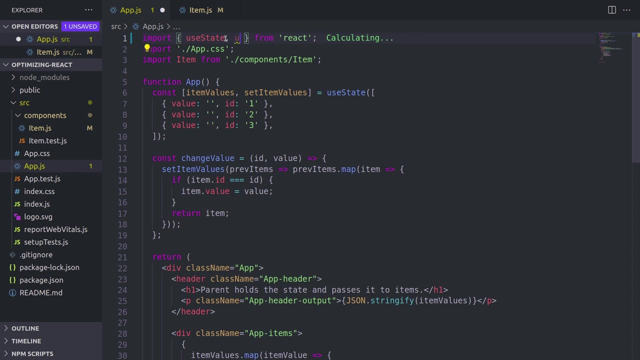 It doesn't. That's why we need to make sure that it somehow stays in the memory. Well, not literally in the memory, but keeps the same reference. Well, for that we can use the hook. It's called useCallback. It works very similar to memoizing. 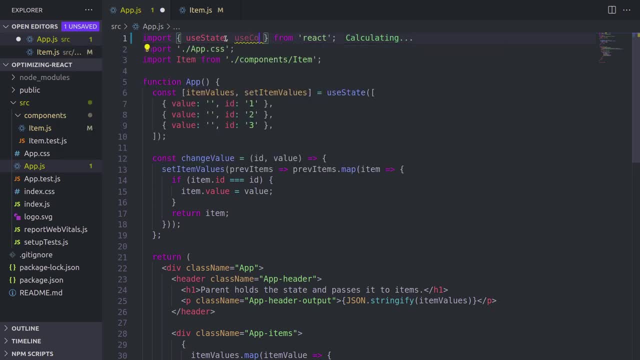 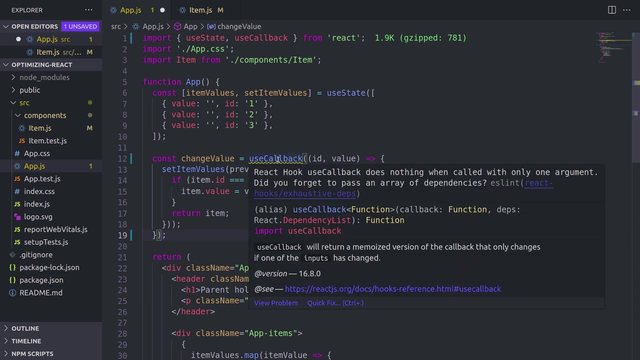 So useMemo, although it doesn't work with usual props, but it works with functions. So I'm going to import useCallback now, And what we do is we simply wrap our change value function with useCallback. Okay, something is wrong. There's a yellow underline. 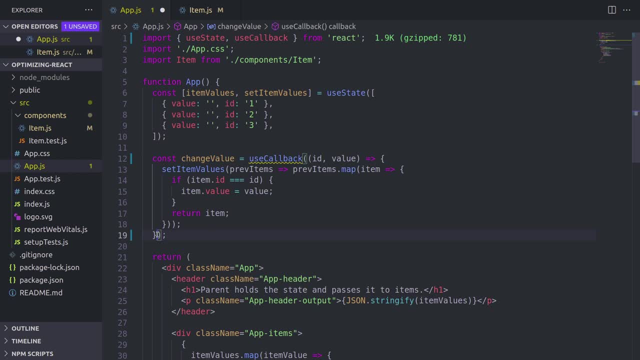 Let's see. Did you forget to pass an array of dependencies? Well, apparently useCallback works. It's very similar to useEffect, so it expects an array of dependencies. In our case, we don't have any dependencies. We simply wanted to kind of memoize the function. 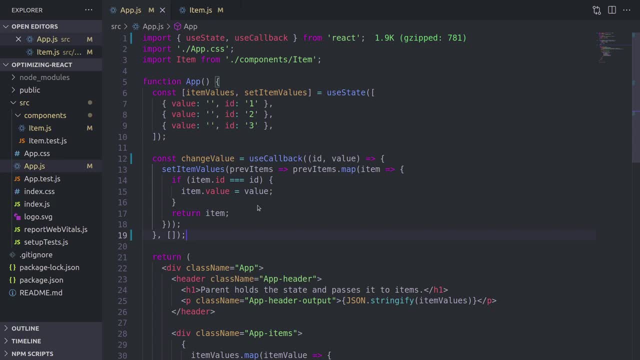 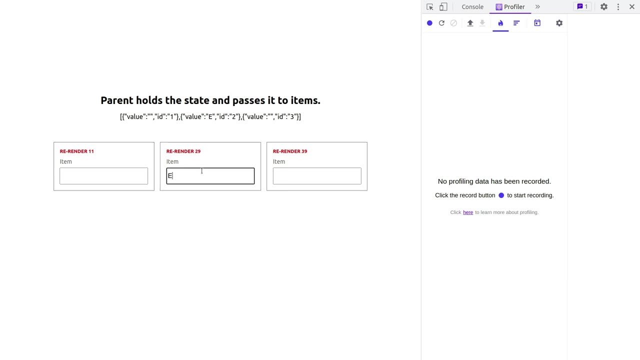 So we pass an empty array And now let's get back to our app and we're going to be typing again. But first clear the console and let's change one of the boxes Editing And, as you can see, the re-rendered numbers are not changing. 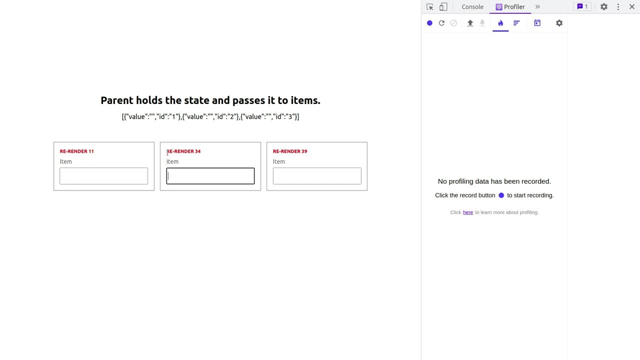 And also there's no outline in other boxes, meaning react-dev-toolscom does not recognize any re-renderings anymore. And that was it. I hope you enjoyed the video And, if you did, please give this video a like. It's going to help me a lot. 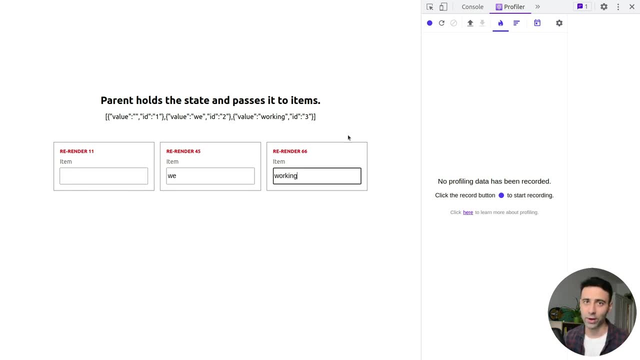 And if you are interested in optimizing your JavaScript code as a whole and you want to find memory leaks in your app, make sure to check this video out. It's going to be interesting, I promise. 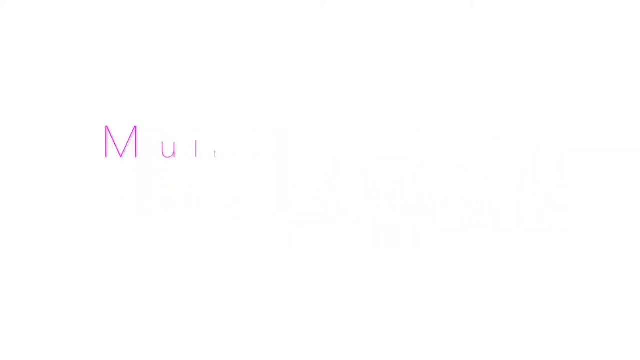 Hi there. so in this video I'm going to be showing you how to multiply 2x2 matrices together. So they're called 2x2 matrices, because there are two rows and two columns in all of these matrices. So when we're multiplying 2x2 matrices together, our answer will also be a 2x2 matrix. 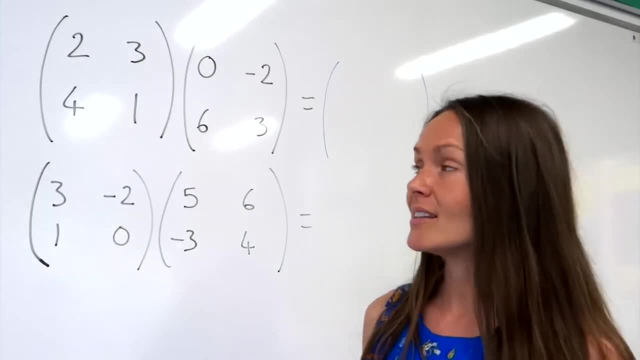 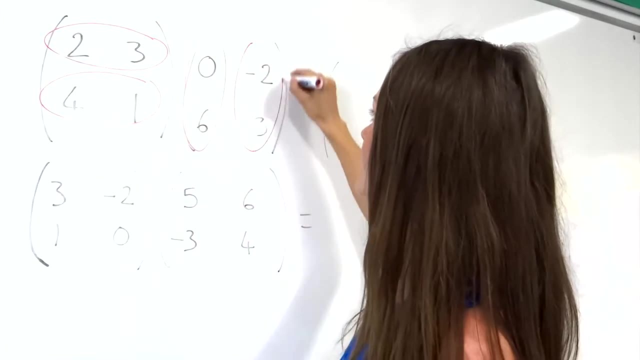 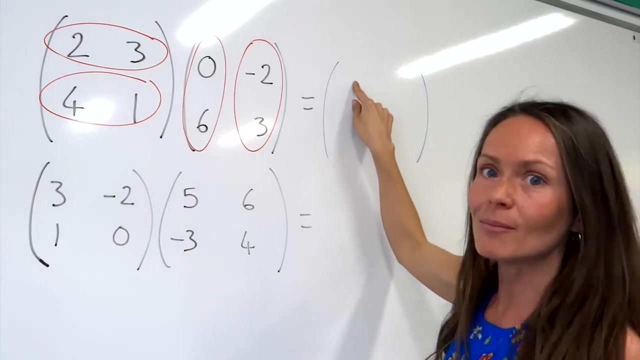 Alright, now, before I start multiplying these matrices together, I'm just going to draw rows around the first matrix and columns around the next one. Okay, and you'll see why in a moment. To find the top left element, so the top left number, in our answer matrix, I have to use the top row and the left column. 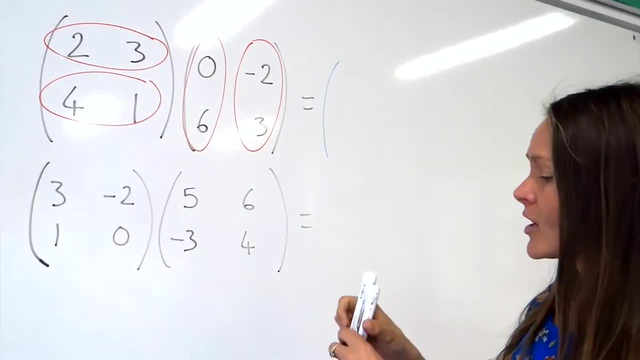 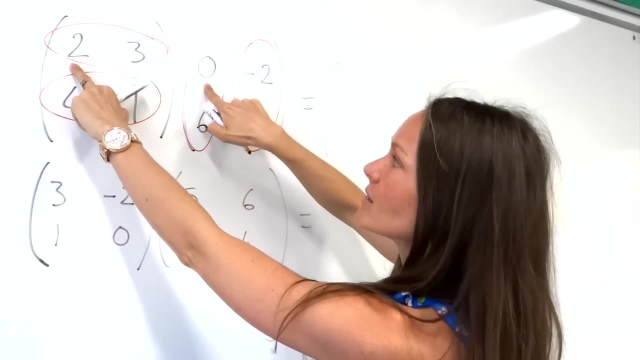 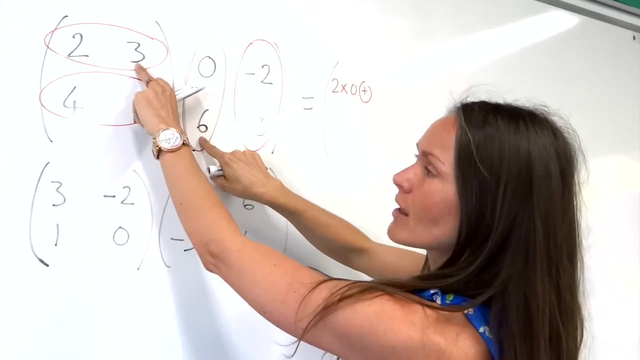 And I'm going to be multiplying, adding these numbers together. So to find the top left one- Remember I'm using the top row and the left column- I multiply these two numbers here together, so 2 multiplied by 0.. And then I add and multiply these two together, so 3 multiplied by 6.. 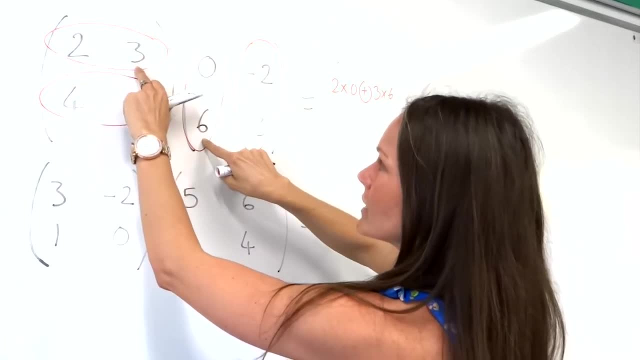 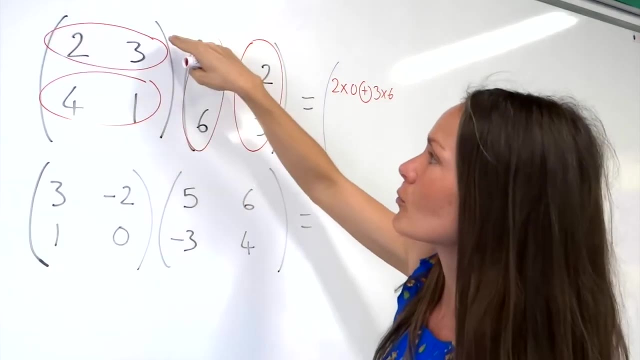 So I'm doing 2 times 0 plus 3 times 6.. Now for the top right element. in our answer I'm going to use the top row and the right column. So again, I multiply, Remember, from left to right and from top to bottom. 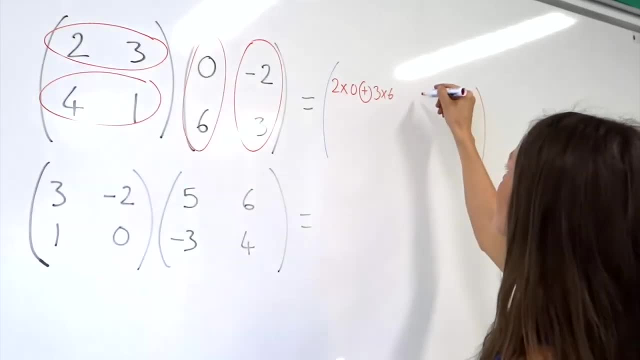 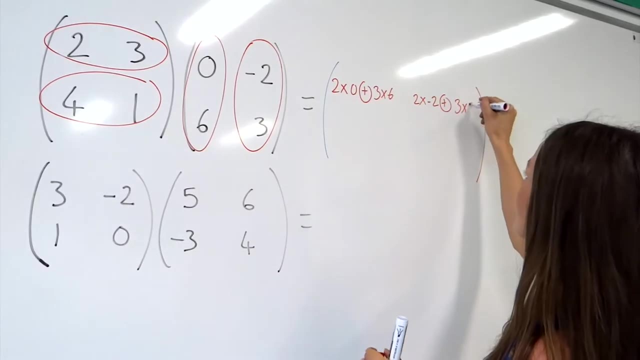 So I'm doing 2 multiplied by minus 2, and then plus again, 3 multiplied by 3.. Okay, so you're doing 2 times minus 2 plus 3 times 3, going from left to right, from top to bottom.